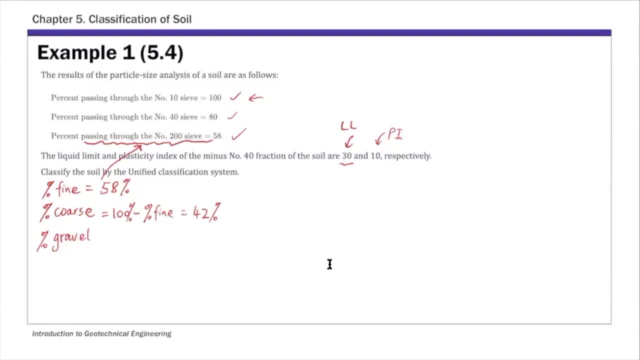 So if you would put number four sieve, it will be put above number 10.. So 100% of the soil passes number four. So this is 0%. So nothing retained above number four. So this means that all the coarse greens 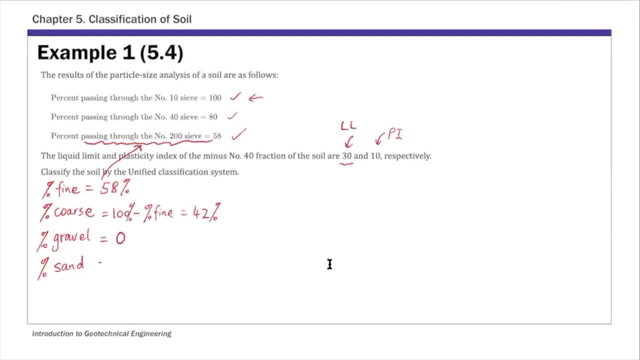 This means our sense. So percent of sand is percent, of course, minus percent of gravel: 42%. So again, let me put a note here. So 100% passes number 10, so that's given. So that means 100% passes number four. 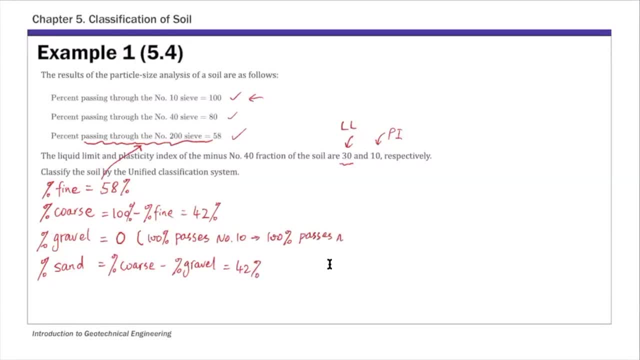 So that means 0% retained on number four, So 0% gravel. And then we have LL and PI, So that's given, And for this example we don't need CU and CC, So that two coefficients are not given. 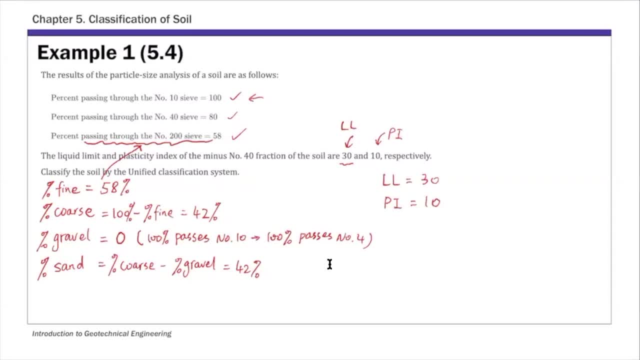 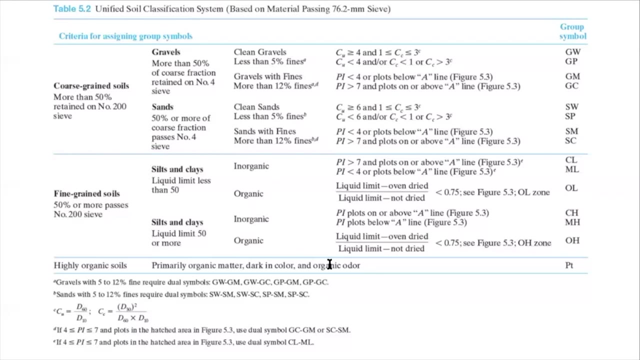 All right. so that's step number one, And then let's use that table 5.2 to determine. So, table 5.2, as I mentioned, we enter from the left-hand side, So enter from the left And the first split here. this is that- two broad categories. 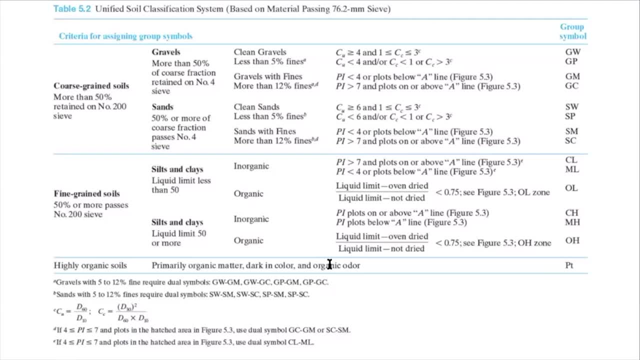 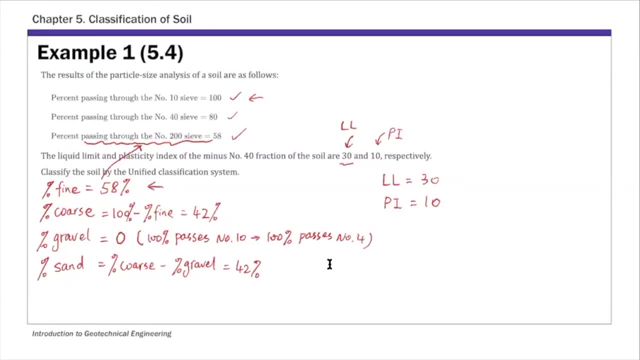 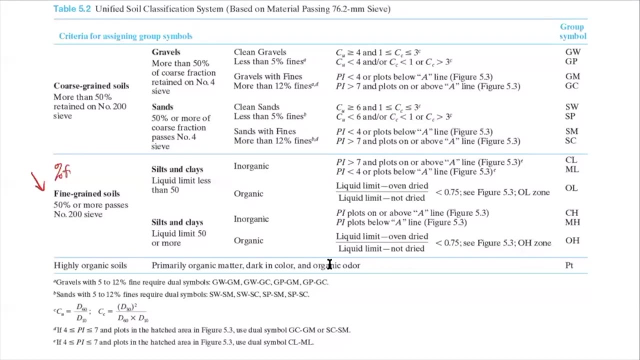 For our soil example: one percent of fine: 58. So more than half of the soil is fine. So that means you use fine green soil. So percent of fine, in our case 58%. And then the next are: this is liquid limit. 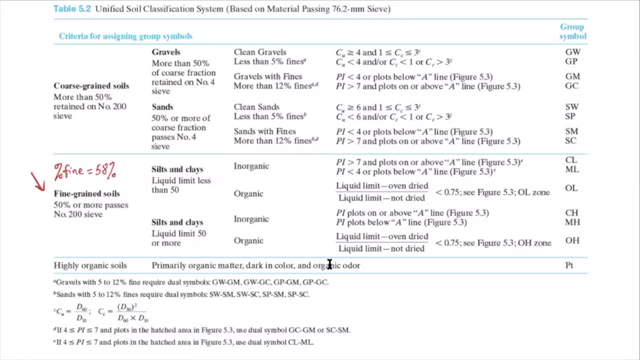 So for this soil liquid limit is 30. So it's less than 50%. Our soil liquid limit is 30. So that's why we pick this liquid limit less than 50 route, As I mentioned, unless it's explicitly given. 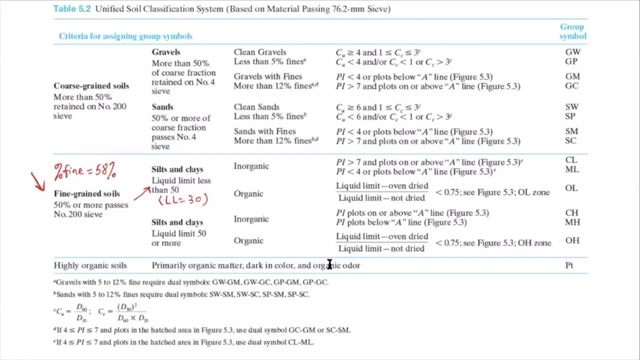 we're going to assume all soils are inorganic in this course. We're going to go this path And the next is that PI For this problem PI is 10.. And then we also need to check if it plots above A-line. 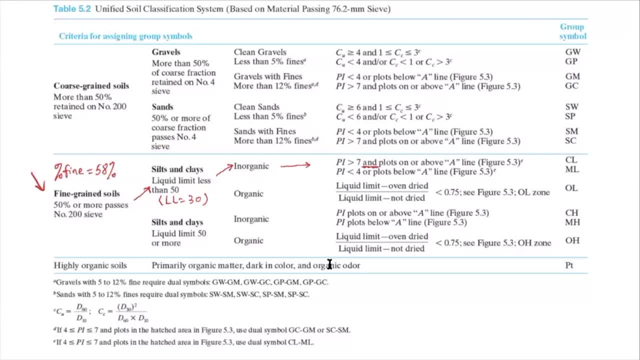 There's an and here There's an, and So you need to meet both criteria. And then we also need to check if it plots: above A-line There's an and here There's an, and So you need to meet both criteria. 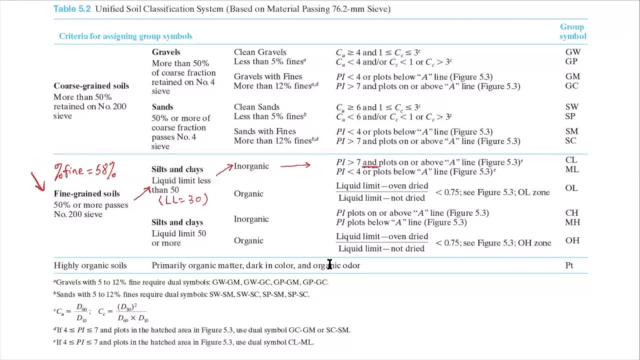 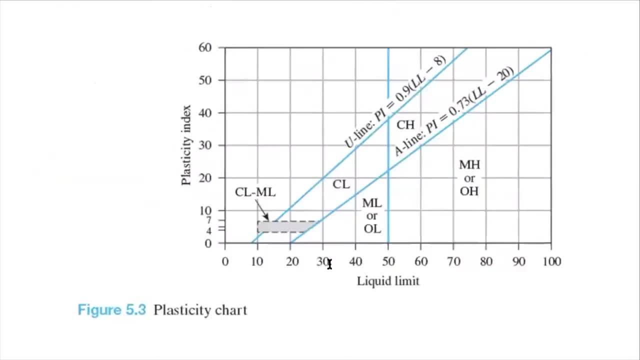 So you need to meet both criteria If you want to pick CL, So PI greater than seven. we meet that, And then let's plot this soil on the plasticity chart. So for this soil LL is 30. And PI is 10.. 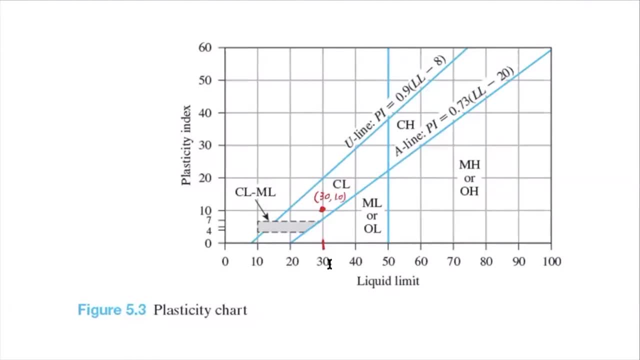 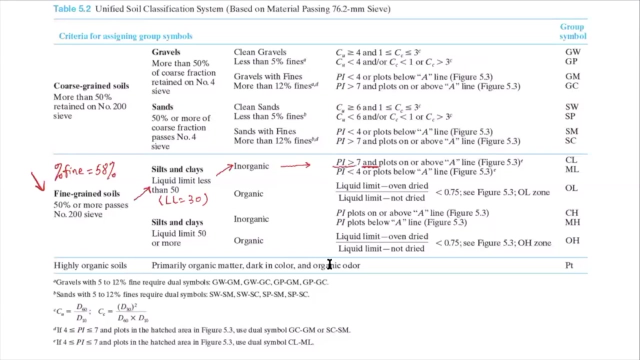 So that's our soil, That's where it plots on this plasticity chart And this is clearly above A-line. So this soil is above A-line, above A-line. So that means we meet both conditions. Pi is greater than seven. 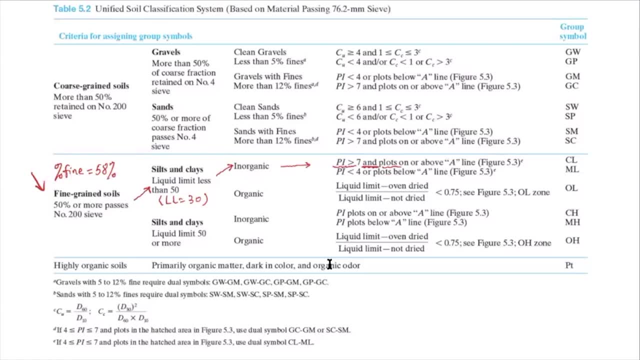 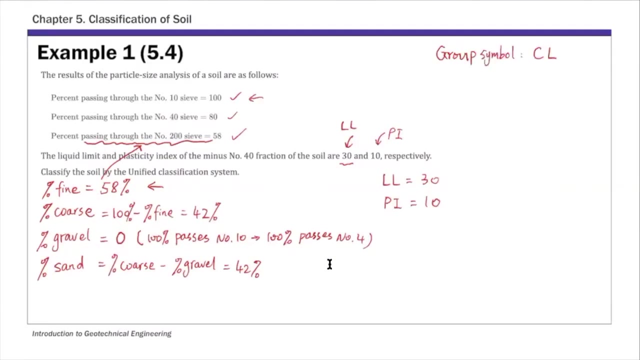 and the soil plots above A-line, And then the group symbol CL. Okay, so that's a group symbol. Remember, that's just one part of the classification. A complete classification needs both symbol and name. So let's find out the group name. 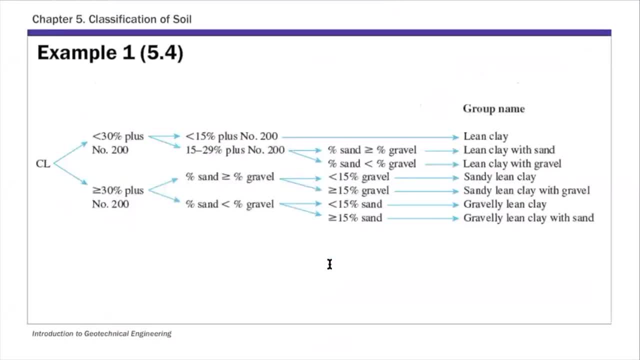 For group name, we're going to use that group name chart And for this particular soil, we're going to use this figure here. So this is a part of that, figure 5.4.. And we start from the group symbol. So we have found that this group symbol is CL. 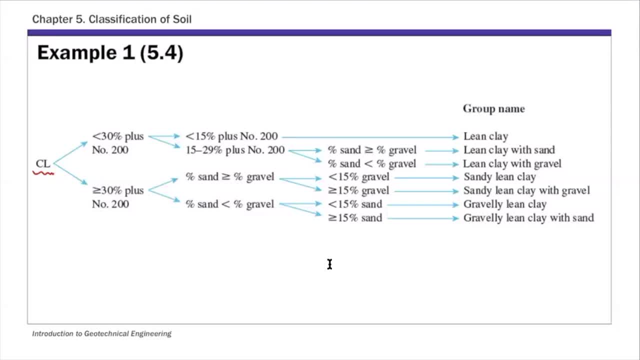 And then, for this soil, let's look at the percentage of fine, Remember. so percentage of fine is 58%. Percent, of course, is 42%, And if you look at these two conditions here, as I mentioned, plus number 200,,